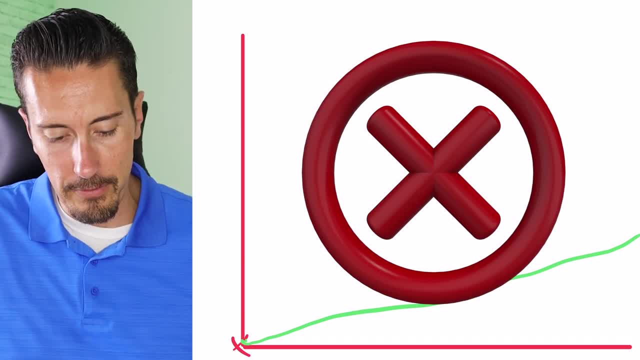 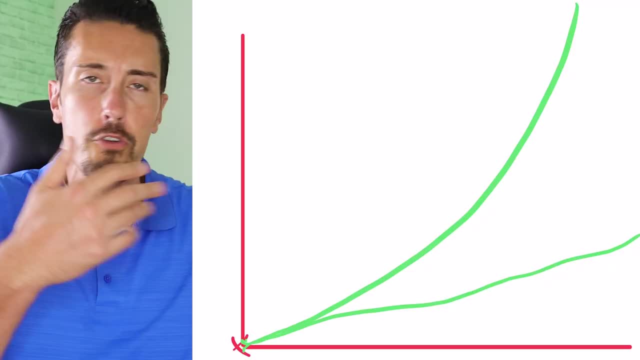 that's not how it works. That's not how compound interest works, Believe it or not. it's more like this: What a huge difference. And it's not a scam. This isn't some alternative investment or crypto that just came out or anything like that. This is just basic math. 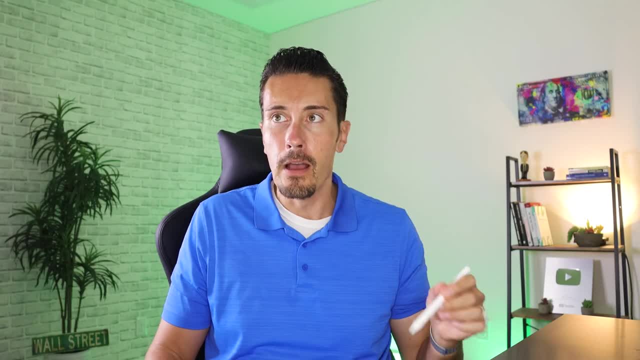 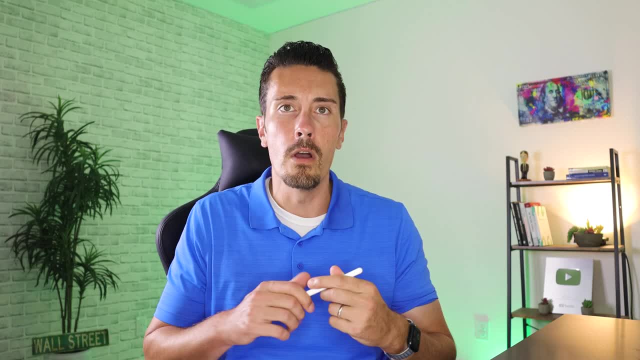 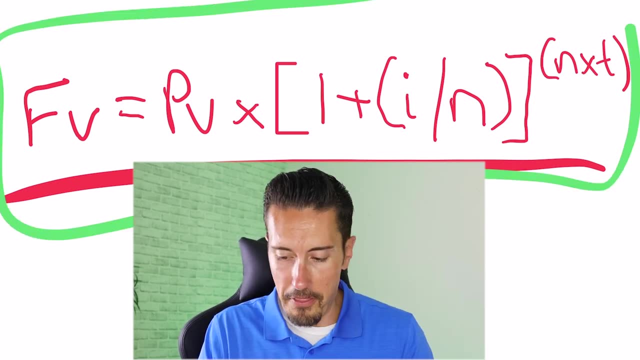 We can get started here today, And I'm going to give you all the details that you need to know with the power of compound interest. Now, as I showed earlier, this is the formula right here. this right here, I mean, first of all, when I look at this, all right, when I look at that. 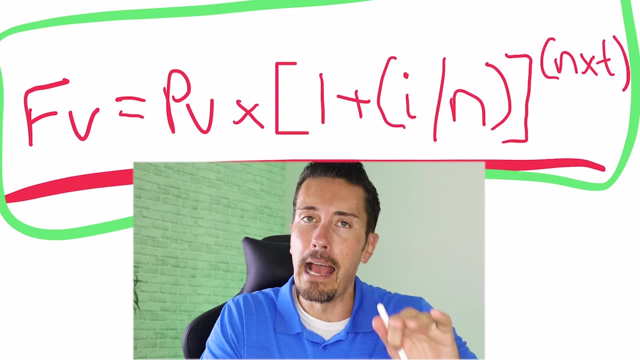 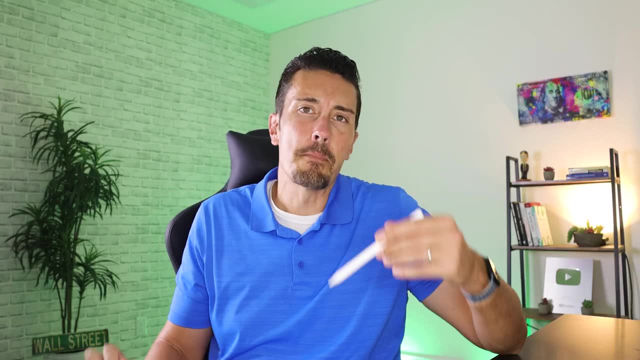 I think, oh my God, math, I hate math. And so how do we like decipher this and make it a lot easier to use? Well, hello Google Sheets. I took the pain and agony out of this Wong formula and I plugged it into Google Sheets that you just plug in your numbers and it'll automatically. 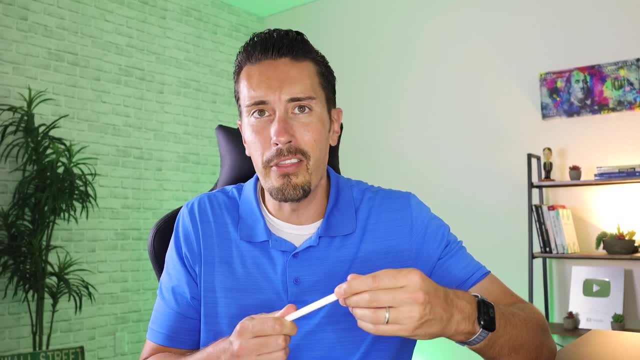 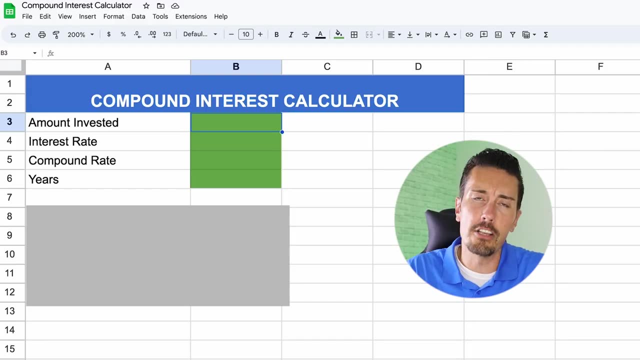 calculate for you. It took me some time because I don't like math. The only thing I ask is: please like the video. I would appreciate it if you find this valuable. So what we're going to look at is how much money you're going to invest. That's the first box, right. The interest rate is how much. 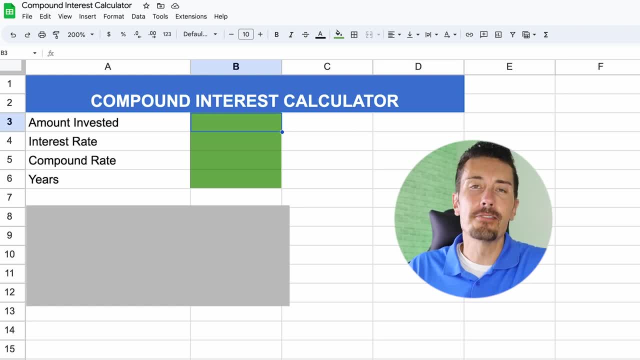 your investment is going to grow over time- The compound rate and the years I'll also explain. but let's just say we're going to put in $10,000. And you know, I think about if we could get a gift from grandma, maybe after we graduated high school and we actually did this. just wait to see. 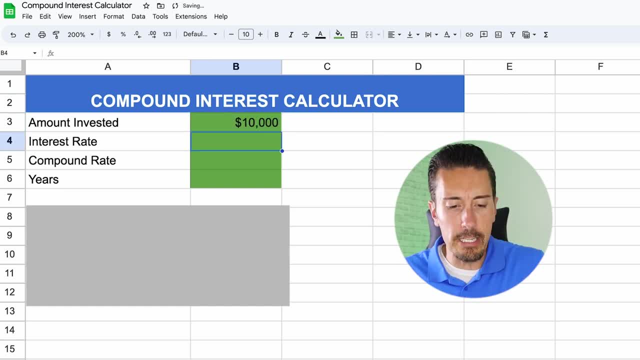 where we would be today. I'm going to plug in the $10,000.. I'm going to plug in the $10,000.. I'm going to plug in the $10,000.. The interest rate: I'm going to use 10%. Now a lot of people ask me why. 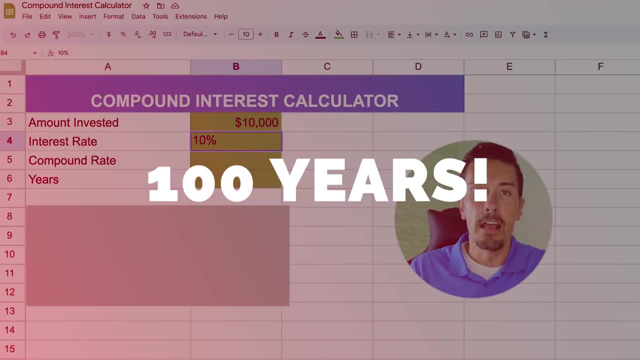 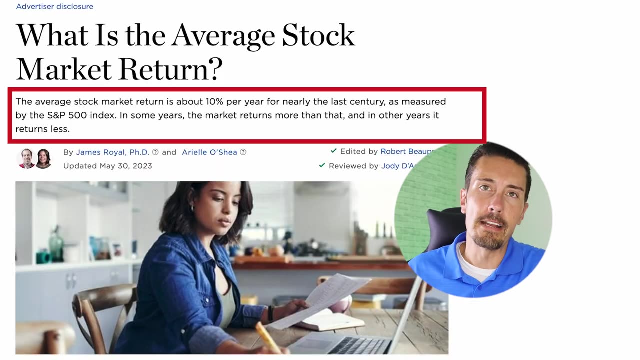 10%. Well, it's because over the last 100 years, the stock market has grown an average of 10% per year. Sometimes it's going to be more, sometimes it's going to be less, As you can see right here. 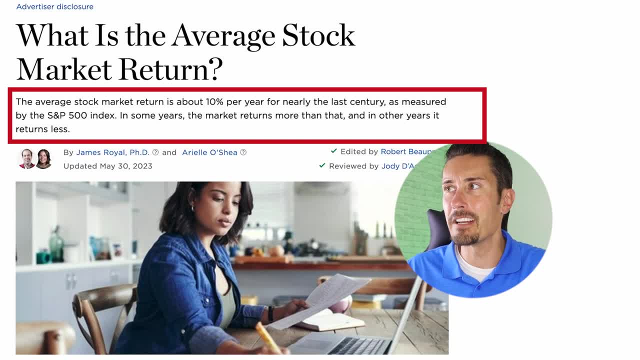 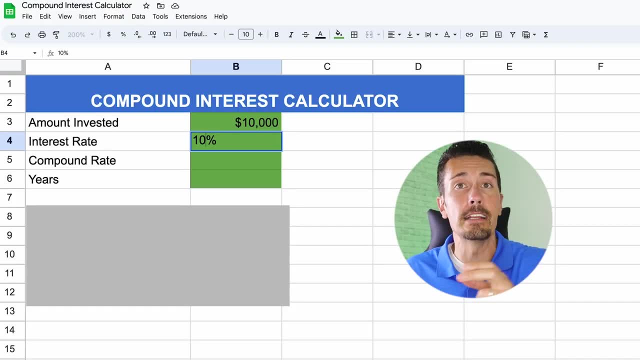 on NerdWallet. the average stock market return is about 10% per year for nearly the last century, as measured by the S&P 500 index. That is why I'm going to select 10%, because we're going to put our money into the stock market, not into some piggy bank or something like that. 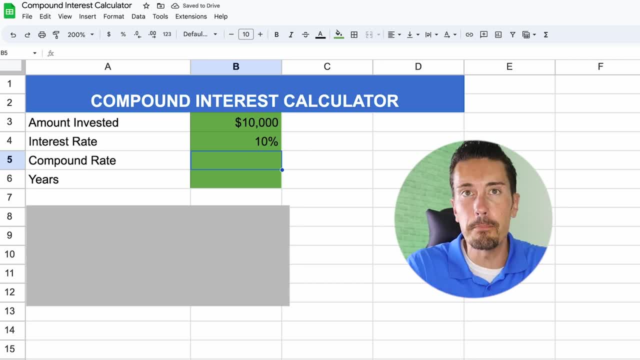 Then the compound rate is: it's going to happen once every year because, as I mentioned, 10% per year, So we would only say one year. And then the key point is: how many years are we going to look at that? Maybe we want to look at the next 10 years, 20 years, 30 years, just for the sake of 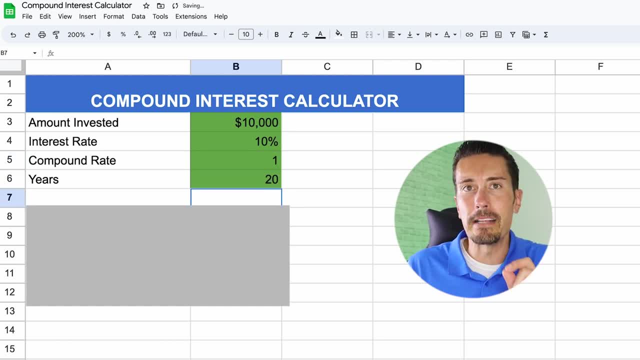 this, let's say, for the next 20 years. Now look at the big difference here. The future value of compound interest will grow our $10,000 to $67,275.. But let's compare that because that becomes even more interesting with the graph that we looked at a little bit. 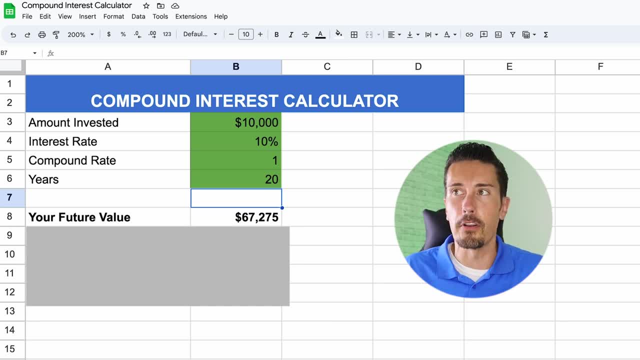 Earlier. most people think it's simple interest, and simple interest is just literally taking that $10,000 and then every year you'll get 10% of the $10,000, which, what's 10% of $10,000? It's $1,000.. 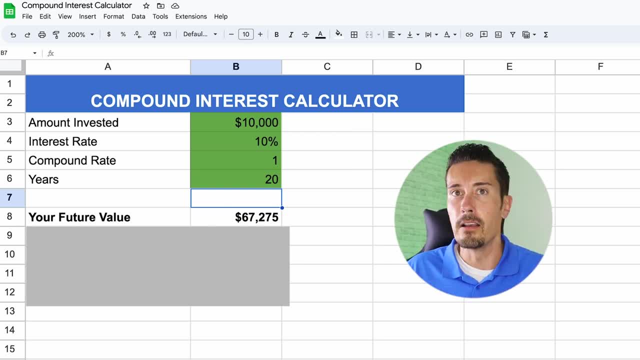 So that means you're just going to get $1,000 every year from here on out. You're not thinking about the compounding effect. So the simple interest value, check that out: $30,000.. What a big difference between what we thought the growth would be and what it actually is Now. 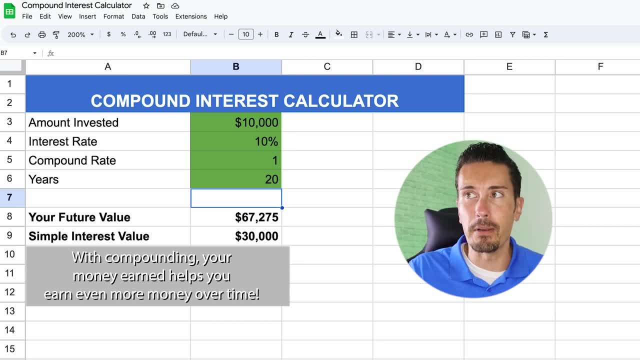 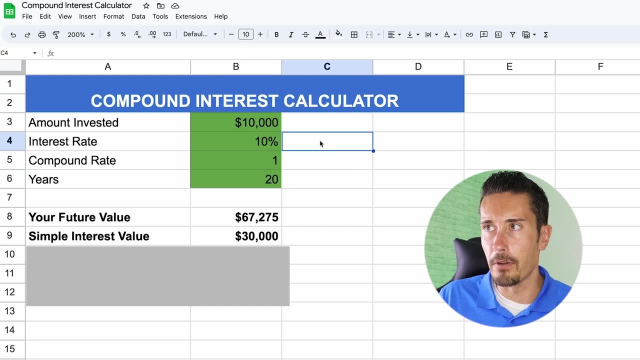 if you already knew this, that's great, But the power of just simply adding in money and letting it grow over time can be significant. In this case, 10% of $10,000,, as I mentioned earlier, is 1,000 big ones, But the difference here is the next year. 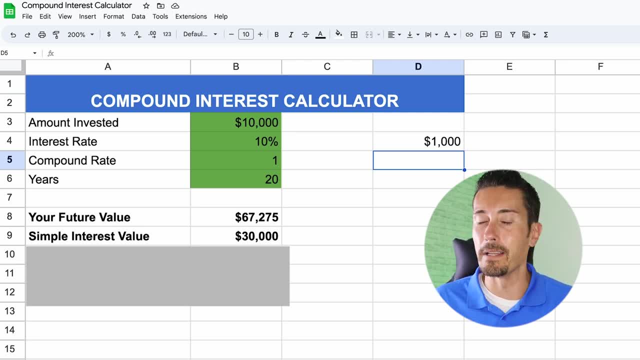 that second year you're not going to get the 10% growth on only $10,000.. You'll get your 10% on $11,000 because you're going to add the $1,000 back in And that's what compound means. So it's. 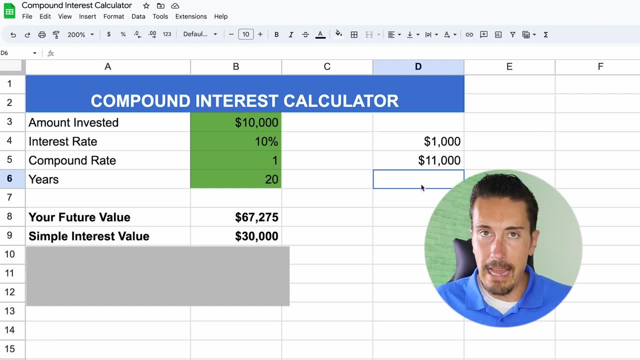 going to take $11,000 and then whatever 10% of $11,000, well, that now goes back into it. Now you have like $12,100, and then that will compound And that's what grows us up to that. 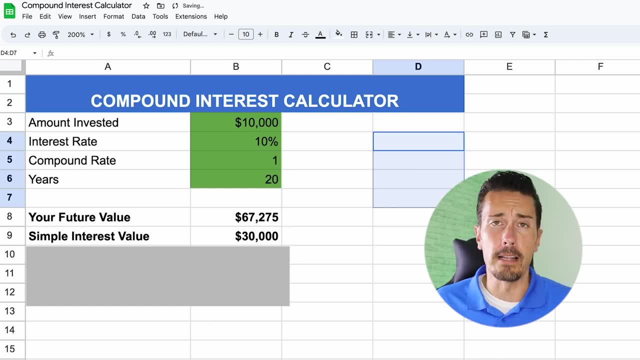 $67,000 in 20 years. But if you're 18 years old, let's say, and you decided to take $10,000.. Now, let's say, you retire at the age of 48. That's your goal. So 30 years from now, 18 to 48,. 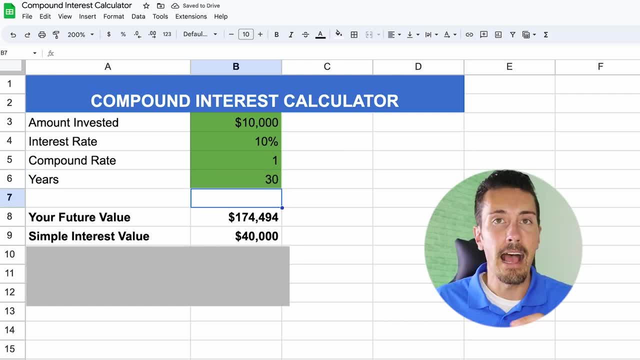 you put in the 30,, you're going to have $174,000 at 48 years old, versus a simple interest value of only $40,000.. Now you might say to yourself: well, wait a minute, I cannot retire on only. 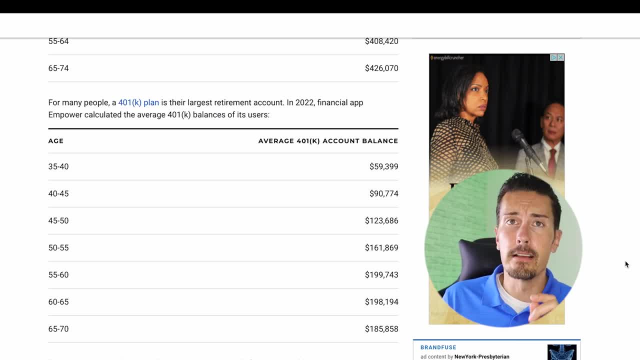 $174,000.. Well, I'm glad that you have that mindset because, surprisingly, according to US news right over here, the average balance at the age of about 48 is only $123,000 as of 2022.. And if we scroll up here to the age of 60, the average 401k account balance is only $198,000.. So either 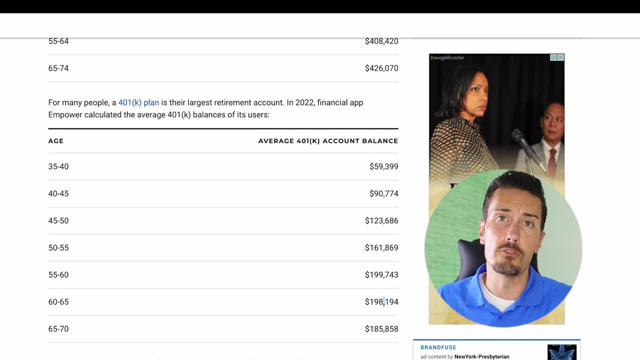 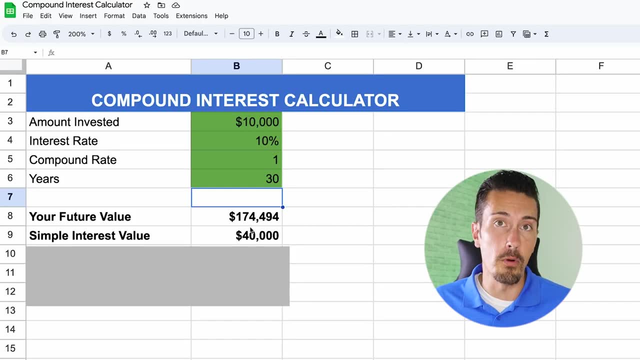 you're going to live off of social security or you're going to hope that you don't have to drain your account that much and live off of that $198,000.. So, going back to our Google sheet, of course $174,000 would. 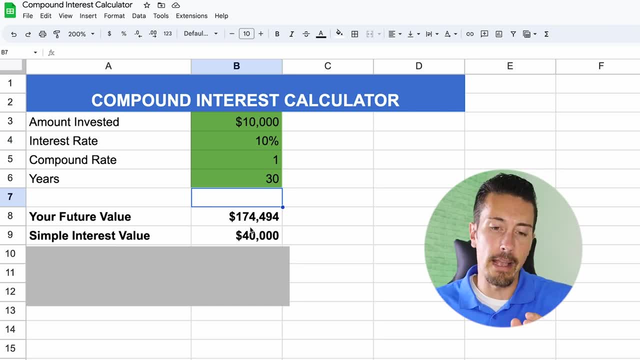 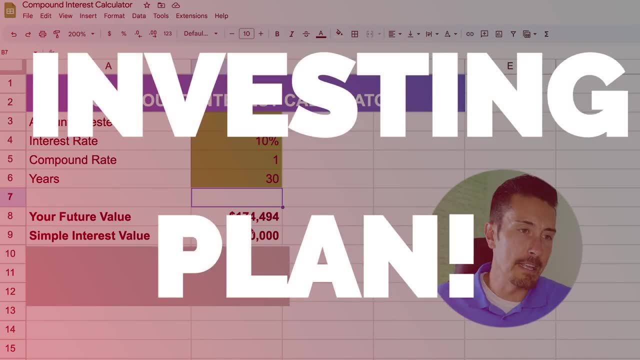 kind of make you average. but you're going to be a little bit smarter and say, okay, I'm going to put my $10,000 of grandma's funds into the account, And then I'm going to come up with an investing plan, Like we talked about in a video last week. an investing plan That's. 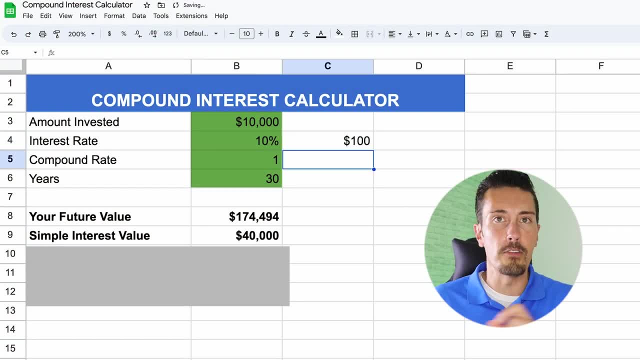 going to say: I'm going to continue to contribute $100 every month from the age of 18 to the age of 48. I'm going to retire before anybody else because all my other friends, they're going to work until the age of 65. I'm going to retire at the age of 48.. Now, believe it or not, 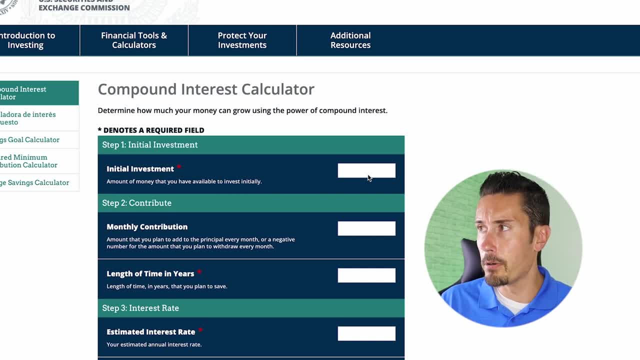 the government is actually doing something good here with investorgov. You can actually put in the same numbers that we just looked at- $10,000, and then the monthly contribution that I mentioned of $100 a month, And what we're going to look at is 30 years, from the age of 18 to 48,. 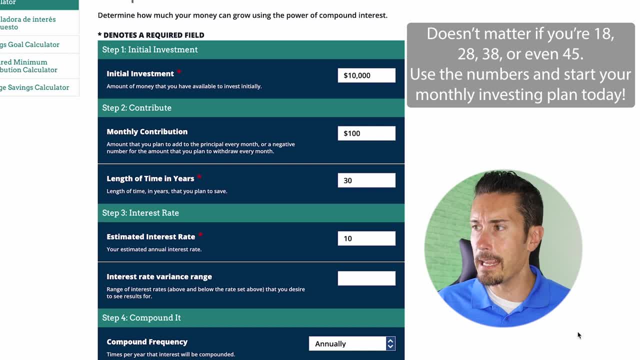 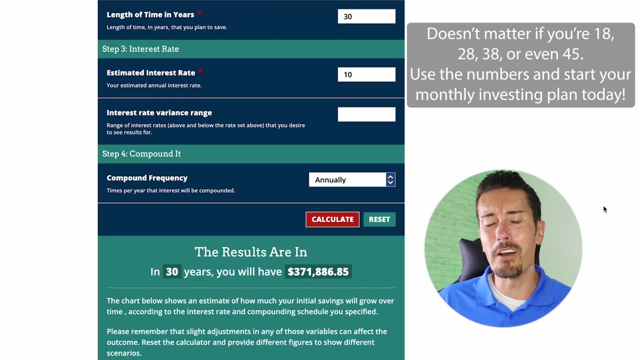 and the interest rate of 10% and it compounds annually. So if we hit calculate, here's what we're looking at. So we're looking at a total of $371,000 now, with a mere $100 a month from that point to the other point. Now what I recommend you do is check out the link in the 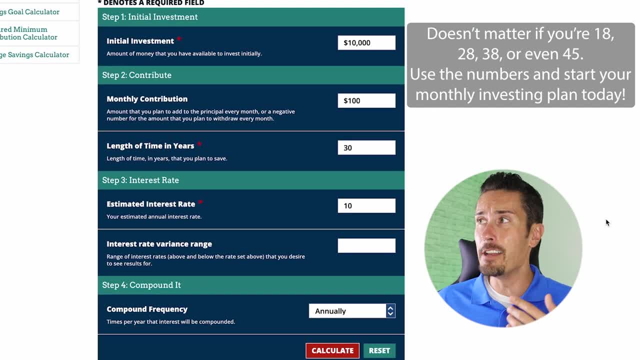 description below I'm going to link to this exact calculator that we're using and you can plug in numbers. Let's say you're not starting with that. Graham only gave you $1,000 to start off, but you're able to put in $500 a month. Play around with these numbers to see. 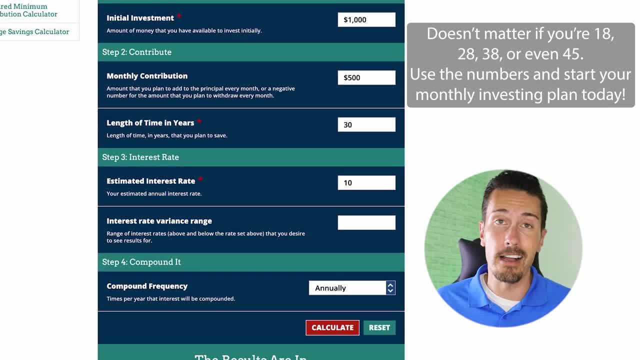 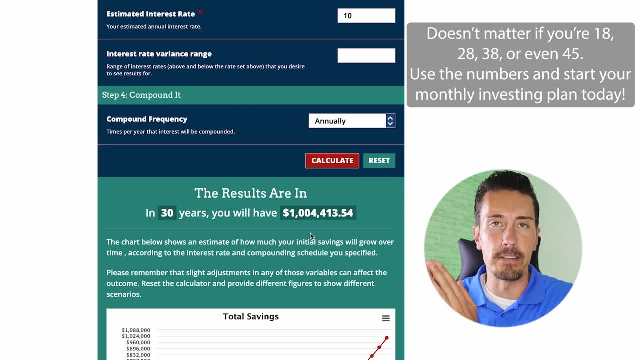 what could happen. You can see right here: at $500 monthly contribution from 18 to 48, wow, you're going to have $1 million. That's beating everybody we just looked at as a result of compound interest. I'll leave you with this fun fact: The rule of 72,. this was actually. 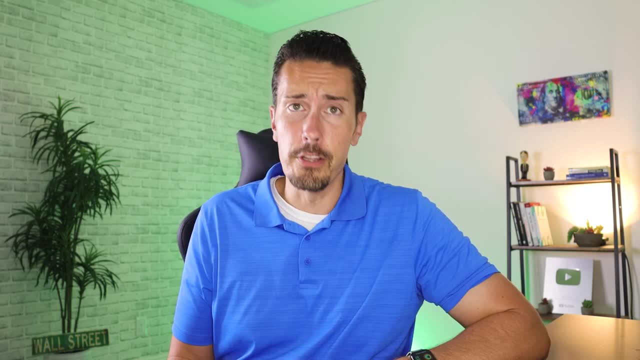 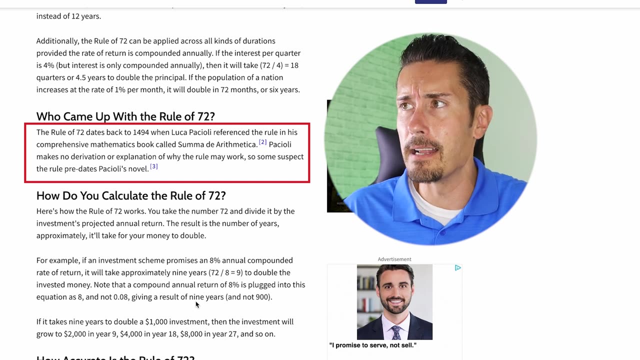 dating back to 1494, so much older than you and I- And it was actually coined by Luca Pacchioli. I don't know if I'm saying that right or not, but he referenced this rule in comprehensive mathematics book called Summa De Arithmetica. I don't know if I'm saying that stuff right again.